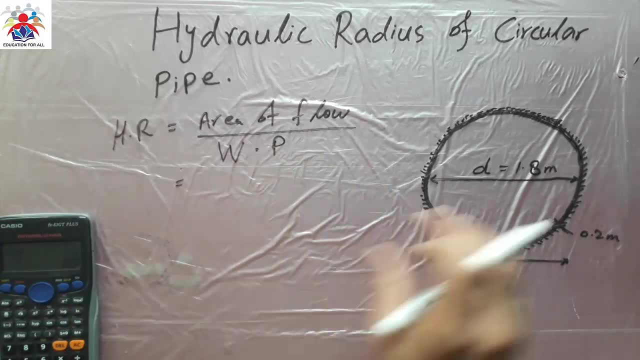 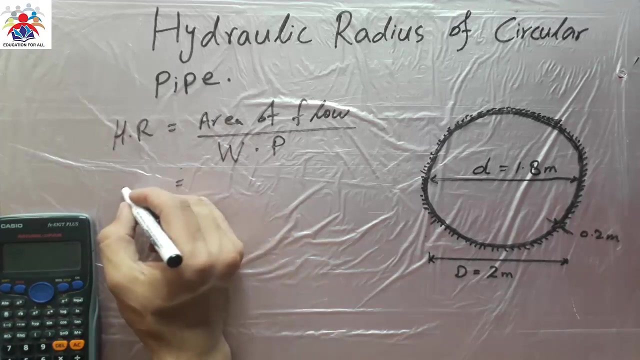 perimeter, So the area of flow. in our particular example, we have to calculate the internal diameter. We have to take internal diameter of our pipe because the water is inside the pipe, So thats why we will take internal meter for this case, our. we are assuming that our pipe is full of water, okay, so 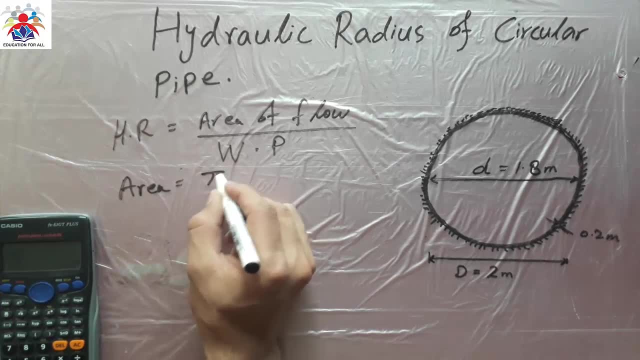 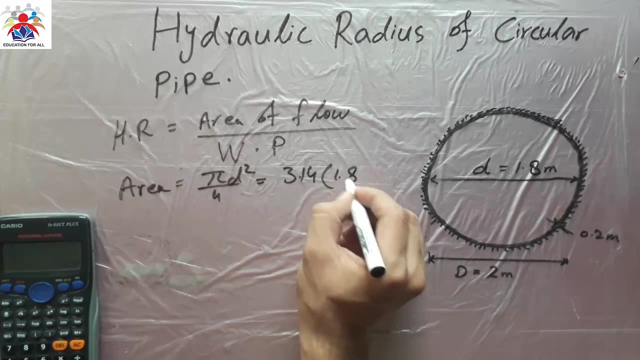 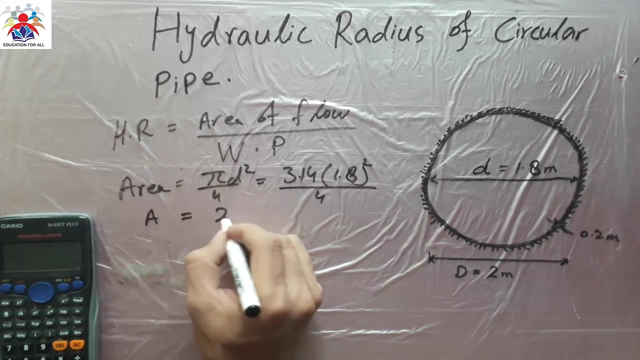 the area would be area of flow would be pi over 4 D square, which is 3.14 multiplied by 1.8 square divided by 4. so we are getting the area 2.54 square meter. okay, so we have got the area. now the main thing is how to calculate. 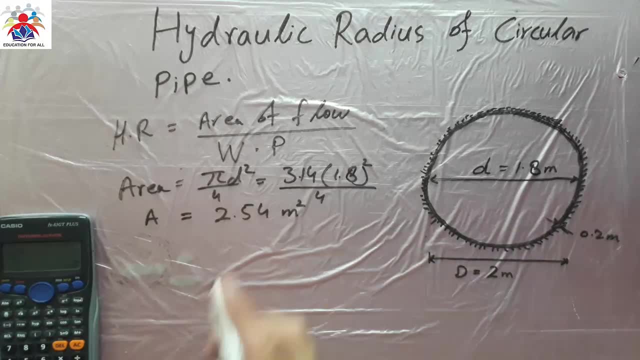 wetted perimeter for circular pipe, for such type of pipe. okay, the wetted perimeter would be: if you just look in the diagram, we have internal diameter 1.8 meter and external diameter is 0, point, sorry. the external diameter is 2 meters. it means that the thickness our, the thickness of our pipe is 0.2 meter. so if 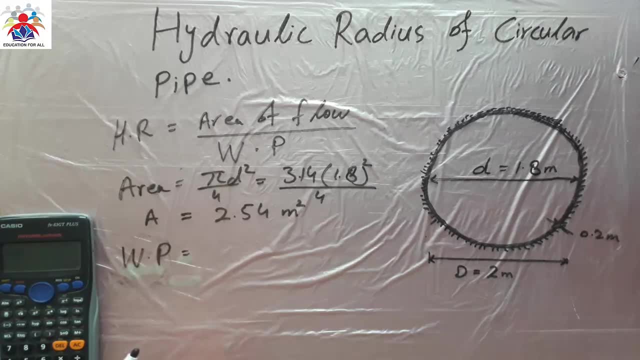 you just imagine where our wetted perimeter would be. obviously it would be a outer edge or outer side of the pipe, so we have to take the external diameter. the external diameter is 2, so our wetted perimeter would be 2 meter in this case. okay, so now we just need to apply a formula for hydraulic radius, which is HR. 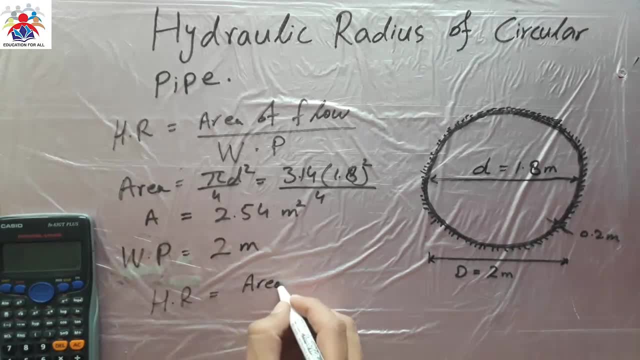 is equal to C. now suppose we have this area divided bylaws ior area divided bywetted perimeter. okay, so the area we have calculated is 2.54 square meter and the wetted perimeter is 2 meters. so what? we will get EMF at used equals, Which is sorry. 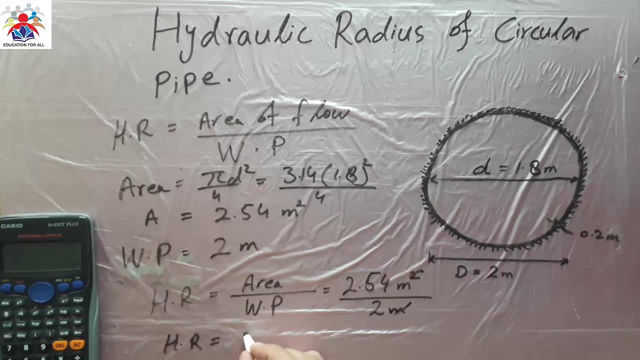 square, cancel out with the meter and we will get one point two, seven meter. so this is our final answer. answer. that's it for today. thank you for watching my video. please don't forget to subscribe my channel.